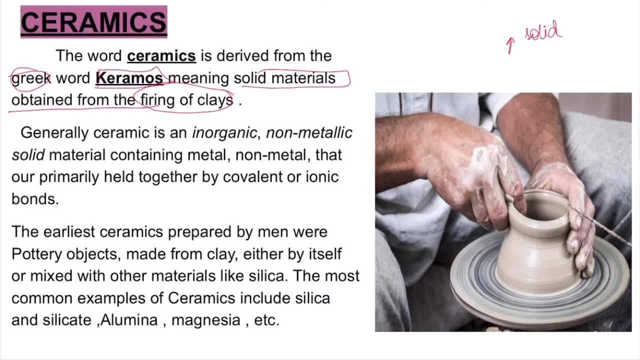 Generally, ceramics are made of solid materials. Ceramic is an. this is the proper definition If we are asked in our exams to define ceramic, so we have to write this: Ceramic is an inorganic, non-metallic solid material containing metal, non-metal that are primarily held together by covalent or ionic bonds. 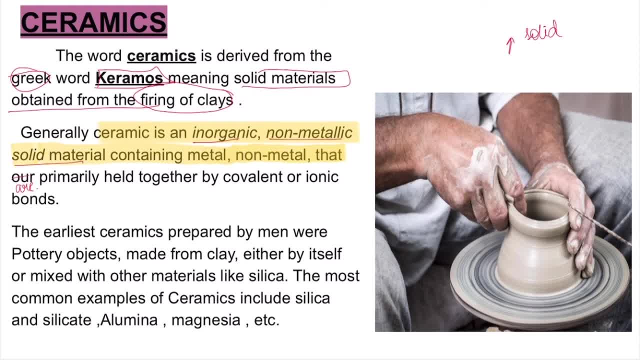 Ceramic is an inorganic, non-metallic solid material containing metal and non-metal. Ceramic is an inorganic, non-metallic solid material containing metal- non-metal that are primarily held together by covalent or ionic bonds. Let us explain one general thing so that it becomes clear what we are studying. 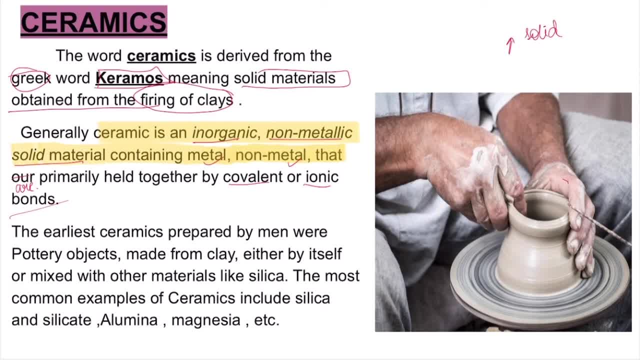 What type of material is ceramics? This picture on the side is what you are seeing. In the ancient times they still made pots with clay and clay. This is very wet. when it was made it was very soft, But as you go on it becomes a little soft. 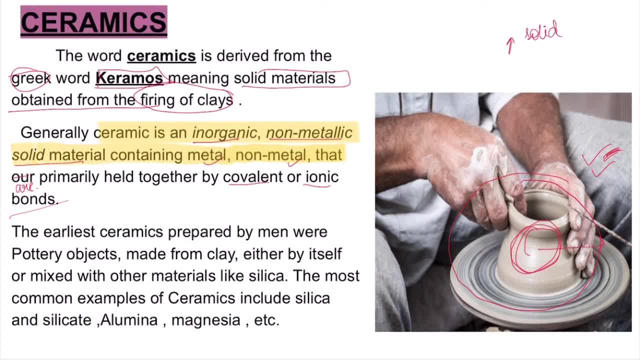 it is dried, it is very rigid. the pots that are used in our house are also made of these. the earliest ceramics prepared by men were pottery objects. this is called pottery right made from clay. these are made of clay either by itself or mixed with other materials like silica. 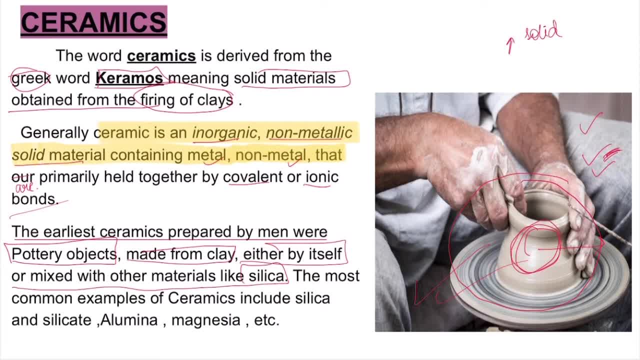 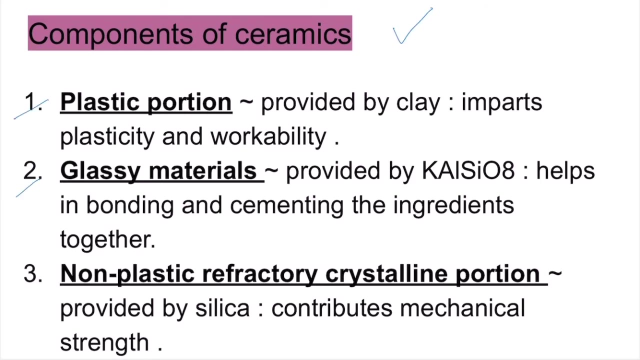 these are either made of clay only or mixed with other raw materials like silica. the most common examples of ceramic include silica and silicates, alumina, magnesia, etc. now we come to the components of ceramics. there are three components of ceramic. first is plastic portion. 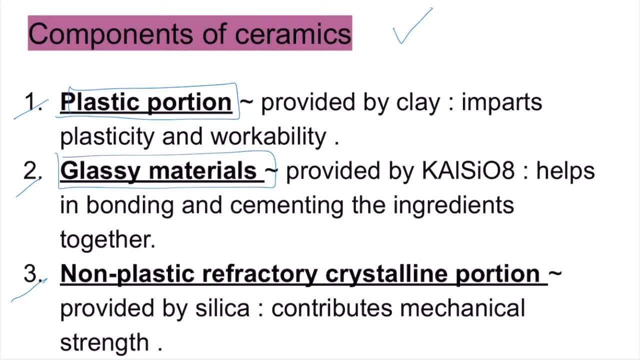 second is glassy materials and third is non plastic, and third is non plastic and third is non plastic: refractory crystalline portion. in plastic portion it is provided by clay. now its work imparts plasticity and workability. glassy material is provided by KALSIO8. 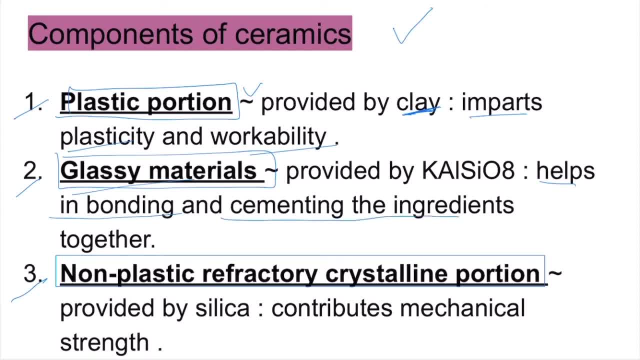 which helps in bonding and cementing the ingredients together, all the things that are used in clay, mix or other ceramics. they have to be joined together. and the third is our non plastic refractory crystalline portion. it is provided by silica, and silica's main work is to contribute mechanical strength. 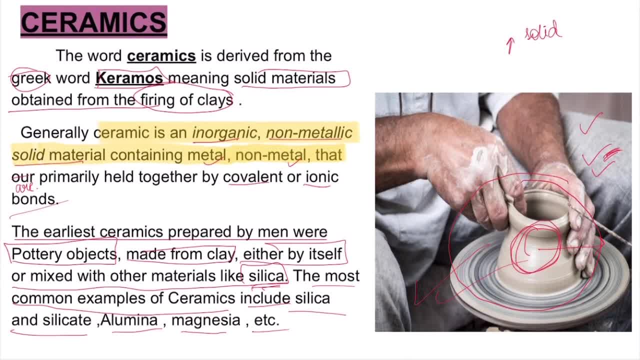 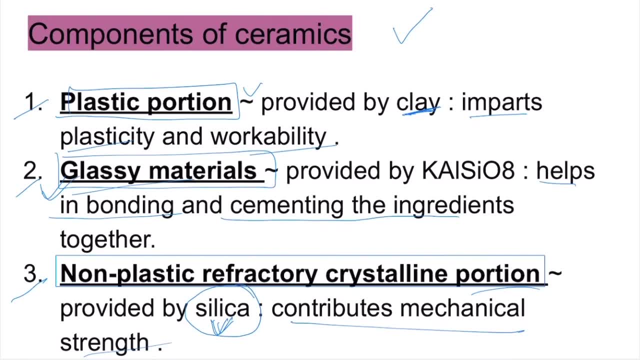 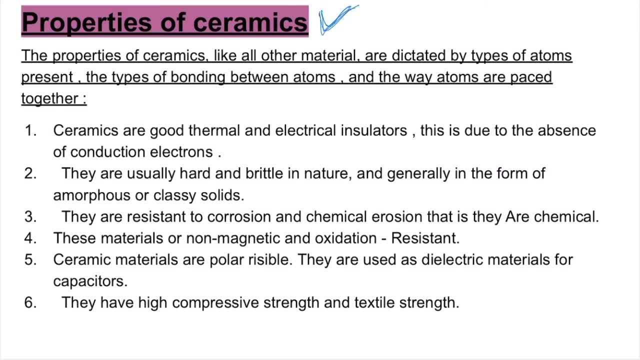 we had read in the back that we mix silica with clay. why silica? because it provides mechanical strength in the material. now we come to the properties of ceramics. this is very important, also from the exam point of view. in the exam it is directly asked properties of ceramics. 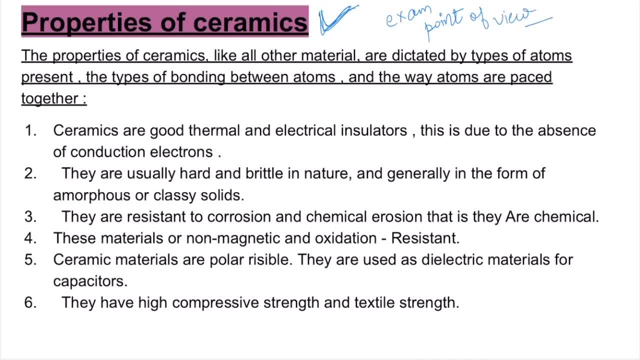 so here we start. the properties of ceramics, like all the other materials, are dictated by types of atoms present, types of bonding between atoms and the way atoms are placed together. any material, how do we know its properties, whether its physical properties or chemical properties? what are the atoms present in it? 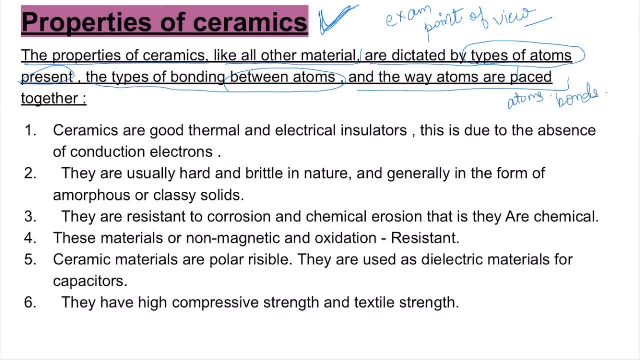 what are the bonds between atoms and how are the atoms arranged? so the first property of ceramics is: it has very easy properties and it is easy to learn. ceramics are good thermal and electrical insulators. why so? because this is due to the absence of conduction in ceramics. 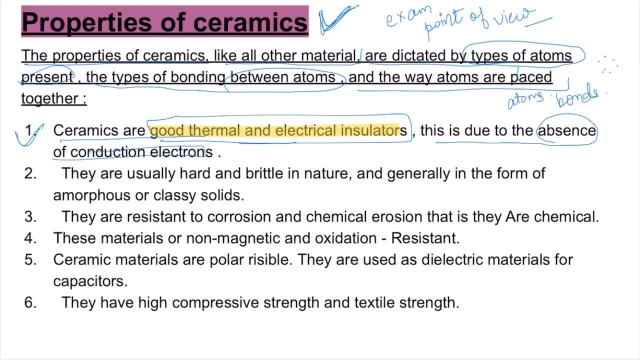 the absence of conduction electrons. they don't have conduction electrons. that's why they are thermally good and they are insulators, not conductors. they don't conduct electricity. second is they are usually hard and brittle in nature. if we take an example of a pot. 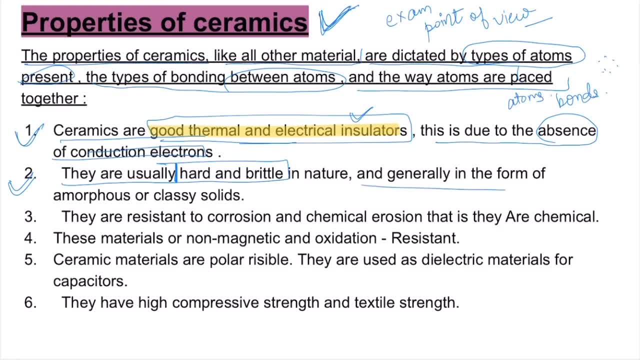 they are hard and brittle and generally in the form of amorphous or glassy solids. it's glassy solids, sorry. third one is they are resistant to corrosion and chemical erosion. they don't have corrosion, they don't corrode, they don't have erosion like corrosion is. if we take an example, 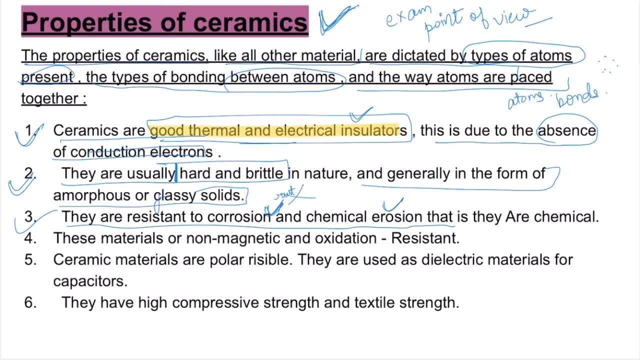 if we apply rust on steel, they don't have anything like that. they don't have chemical erosion. what do we know from all this? they are chemically stable. chemical stable means it is a very useful thing because it reacts with air and water. it doesn't react with anything. 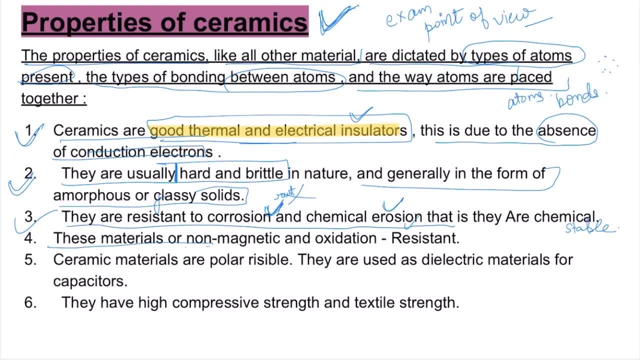 it can be used in many things. these materials are non-magnetic and oxidation resistant. if it is oxidation resistant, then we can keep them in open air without any container. they are non-magnetic. ceramic materials are polarizable. they are used as dielectric materials for capacitors. 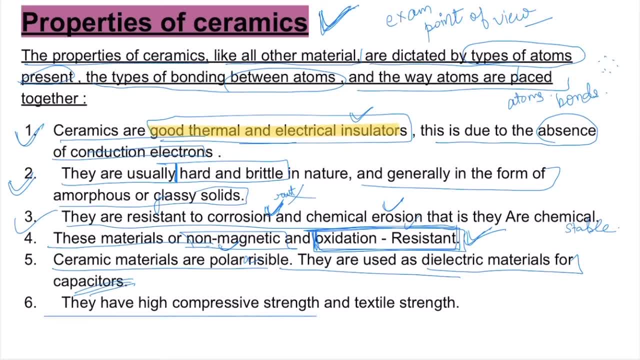 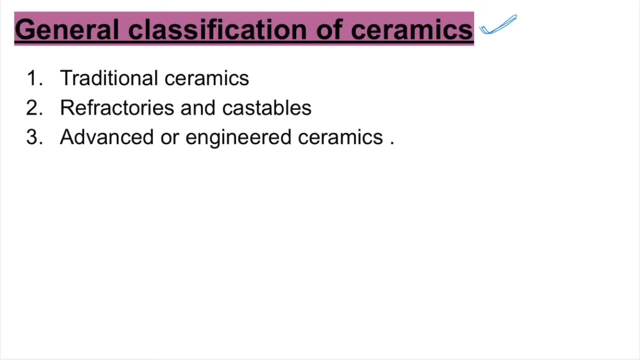 they have high compressive strength and textile strength. these are the six properties of ceramics which are directly asked in exams. they are easy. you can learn them easily. now we have general classification of ceramics. there are three parts in classification of ceramics: traditional ceramics. it is a little important. 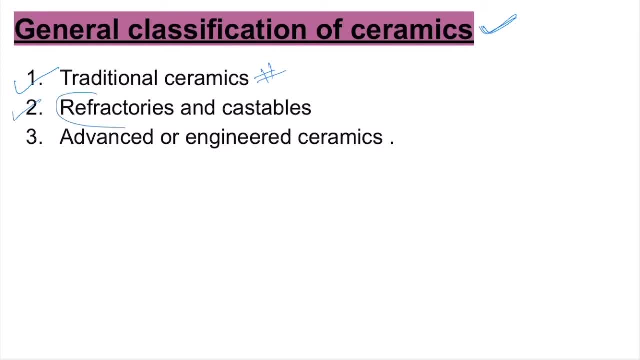 refractories and castables. refractories are a different topic we are going to study in next lecture. and third is advanced or engineered ceramics. among these three, the most important is this, and this is a different topic, we will study this. in traditional ceramics, the raw material is 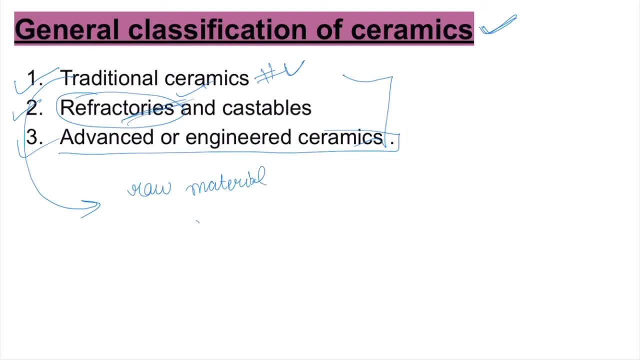 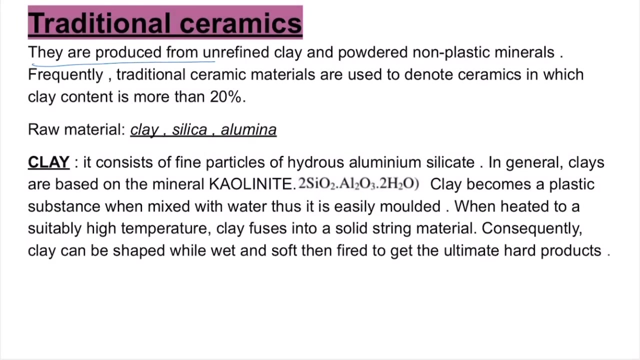 that is clay, silica and alumina, and our advanced or engineered ceramics. the raw material is, that is, silicon carbide and tungsten carbide. we will study about traditional ceramics in more detail. they are produced from from where they are produced: unrefined clay and powdered non-plastic minerals. 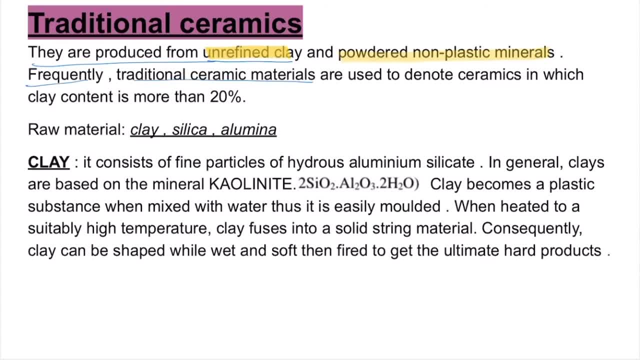 frequently traditional ceramics. sorry, traditional ceramic materials are used to denote ceramics in which clay content is more than 20%. in our traditional ceramics, the clay content is more than 20%. what is the raw material of our traditional ceramics? clay, silica and alumina, among these three? 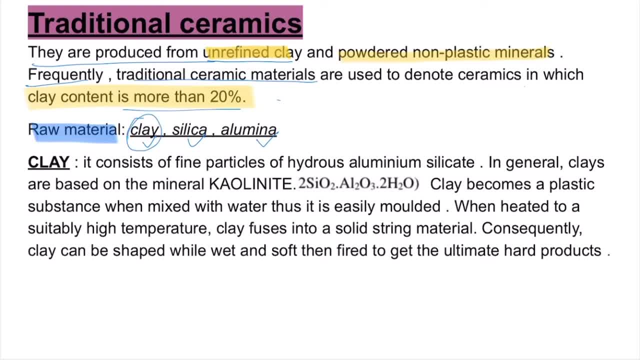 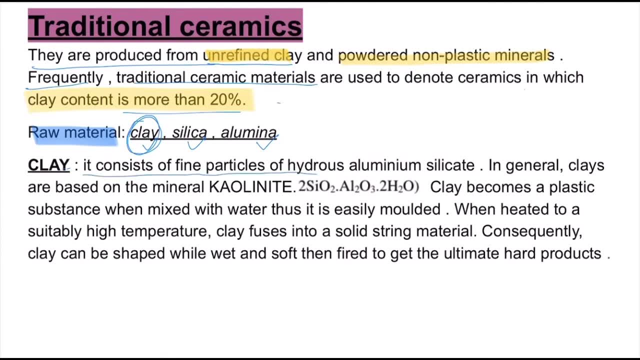 clay, clay. questions are also asked in exams, so we will also talk about clay. so it consists of fine particles of hydrous aluminium silicate. in this fine particles, hydrous means H2O is also present- of aluminium silicate. in general, clays are based on: 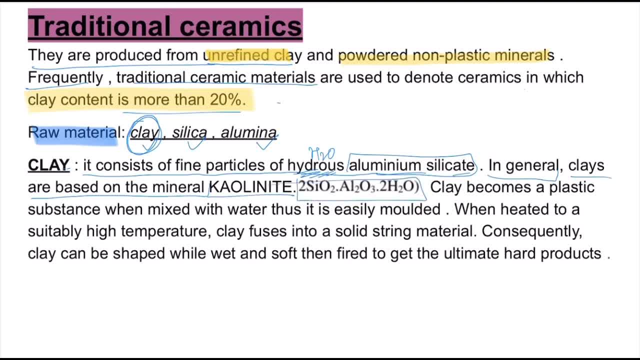 mineral calenite, whose chemical formula is this: clay becomes a plastic substance when mixed with water. it is easily moulded, as we know, we used to play with clay in our childhood, with clay, even in clay. we used to sell clay in the market like stationary shops. 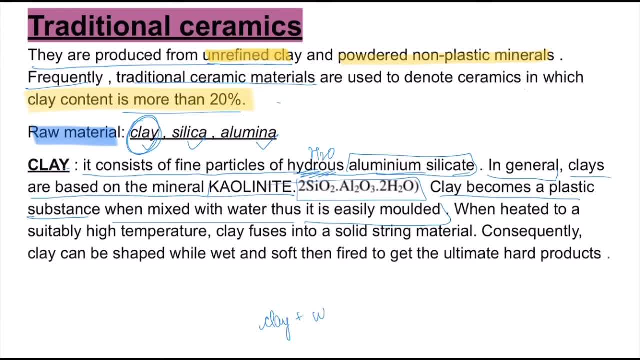 if we wet the clay in clay and put water in it then, and then we keep it to dry for some time, it becomes very hard, and when we put water in clay we can change it in any shape, as we used to play in our childhood right when heated. 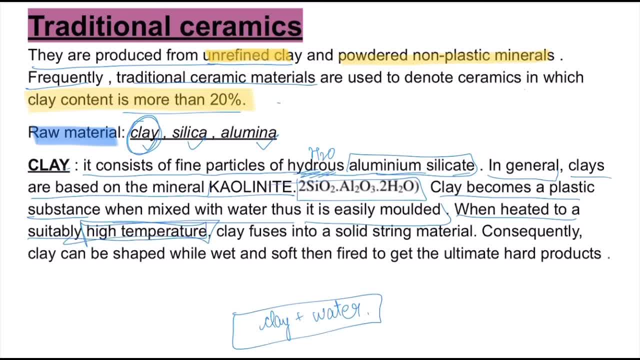 to suitably high temperature. make it fired, like we had read in the first slide, means heat it at very high temperature so that it changes into a solid, rigid. solid clay fuses into a solid, strong material. consequently, clay can be shaped while wet and soft, then fire. 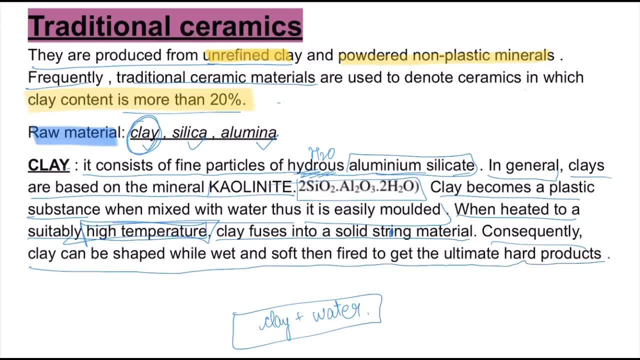 to get the ultimate hard products. as I told you, clay can be moulded in any shape when it is wet, because at that time it is soft, then we can fire it and then we can keep it for a long time means we can keep it under very high temperature. 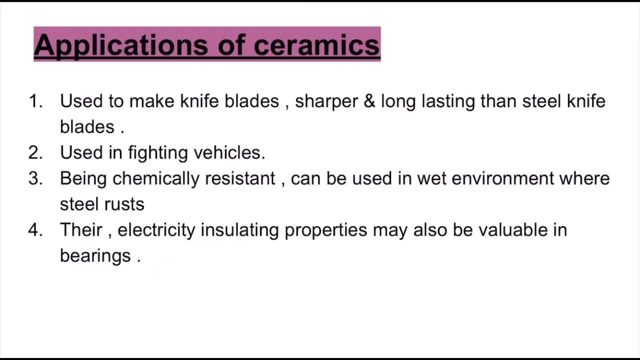 we can heat it so that it changes in hard product application of ceramic. it is also important according to the point of view of exams. the first application is: it is used to make knife blades. these are sharper and long lasting than the steel knife blades it is used in. 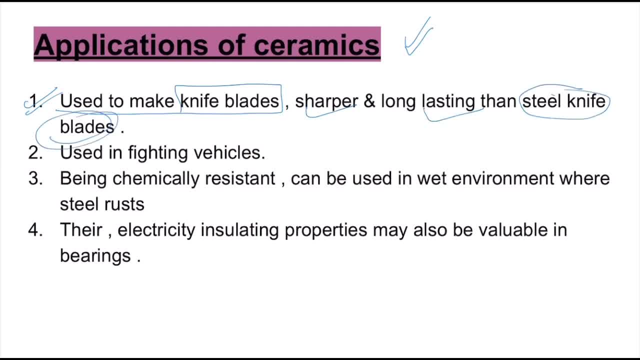 fighting vehicles being chemically resistant. we have read now in this erosion: it is used in the chemical. there is no erosion, there is no corrosion, there is no rust. we have read in the properties. we have read all these. that's why we can use them in wet environment.